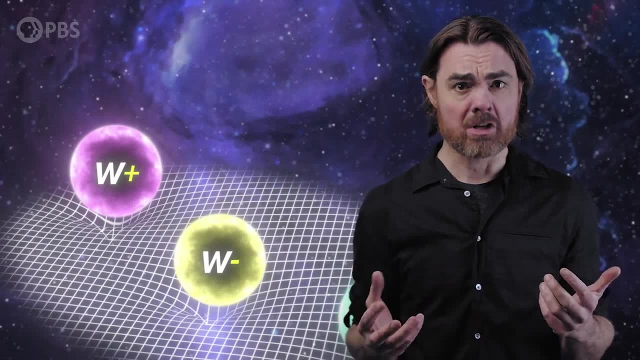 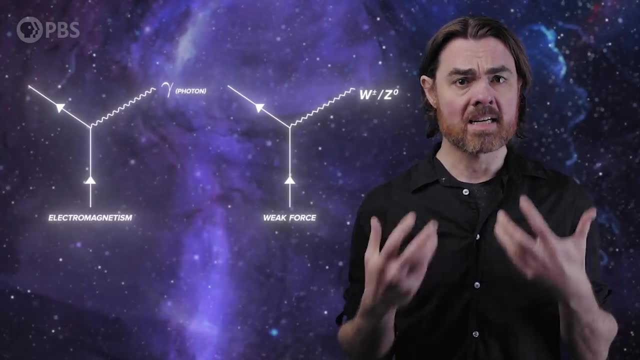 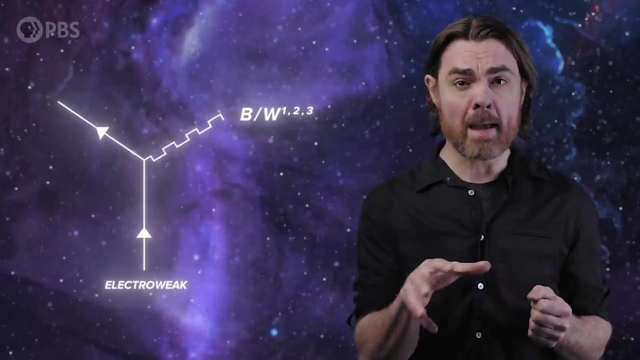 The W bosons are especially weird in that they also have electric charge. This allows the weak force to trespass on the province of electromagnetism, suggesting a connection between the two. This connection hints at a unification of the forces of nature. The path to that unification leads to the Higgs mechanism. 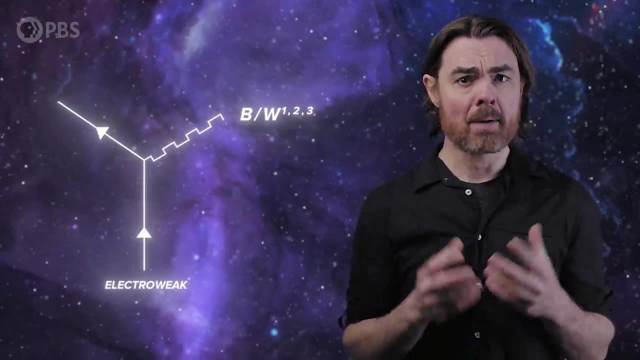 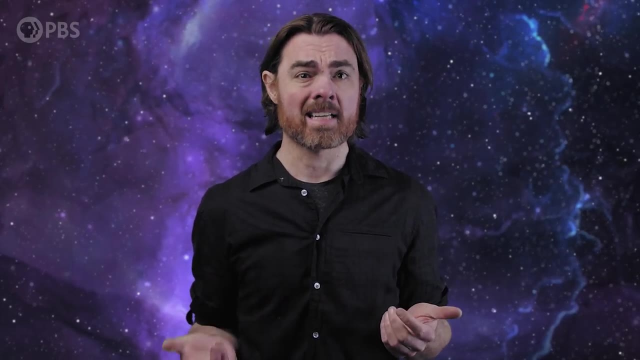 which not only explains the mass of the weak bosons but teaches us about the nature of mass itself. To get to all of that good stuff, we need a bit of a refresher on the episodes that led to this. Fields and forces and symmetries and all that Similar to how the fabric of a drum has. 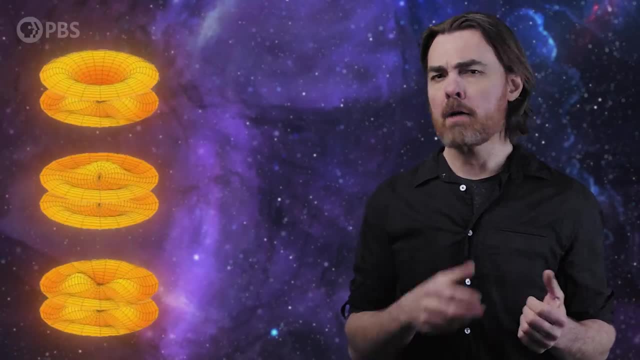 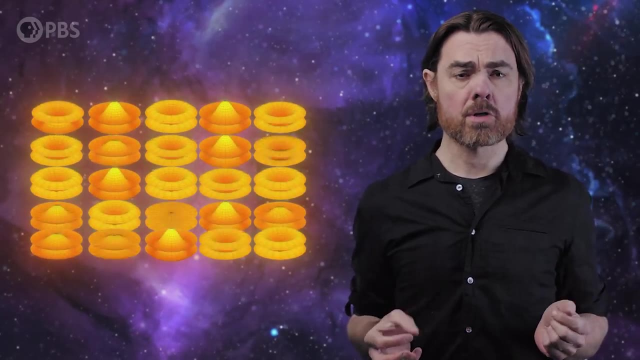 vibrational modes, so does the fabric of reality. Every point in space can wiggle, twist and oscillate in different ways. A quantum field just represents one of these modes. These wiggles are quantized. They come in discrete. 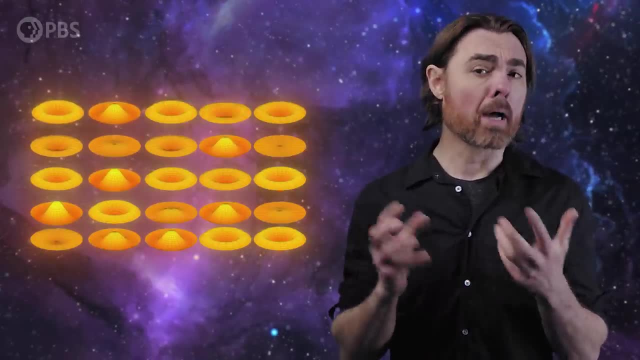 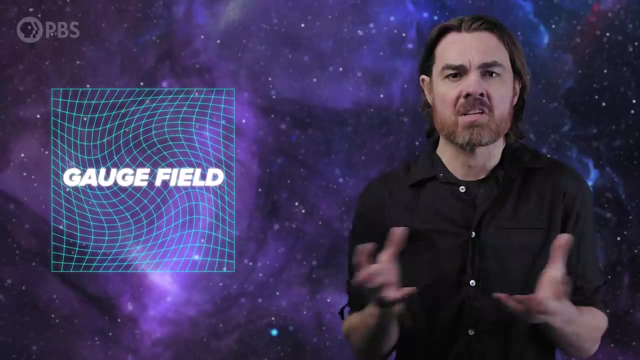 packed with energy that can move around, And those are the particles of the field. One special type of field is the gauge field. These arise from the fact that physics often doesn't care what coordinate system you use. The laws of physics are symmetric under certain. 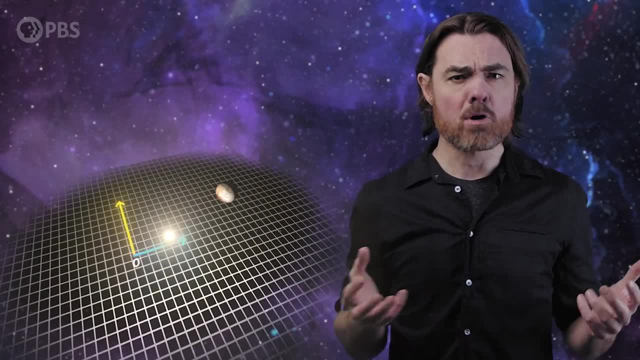 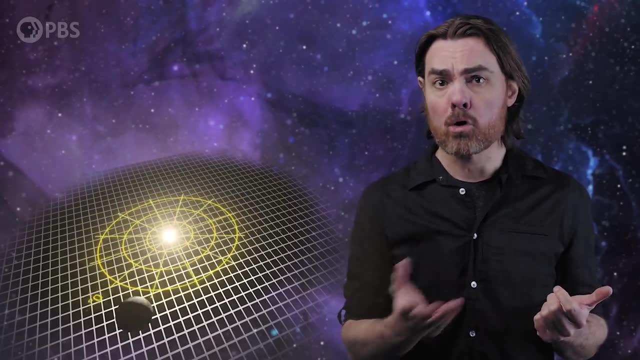 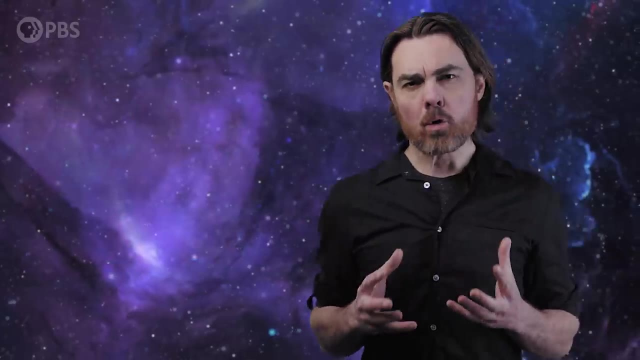 transformations, For example. physics works the same, no matter where you decide to center your xyz axis or where you put the zero point of your angles in polar coordinates. We saw in our episode on Noether's theorem that these symmetries lead to conservation laws In quantum mechanics. this sort of redundant degree. 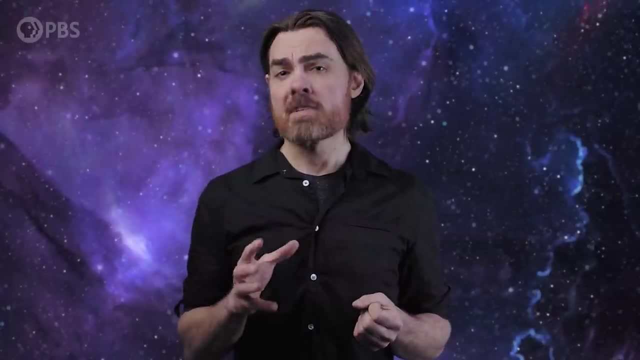 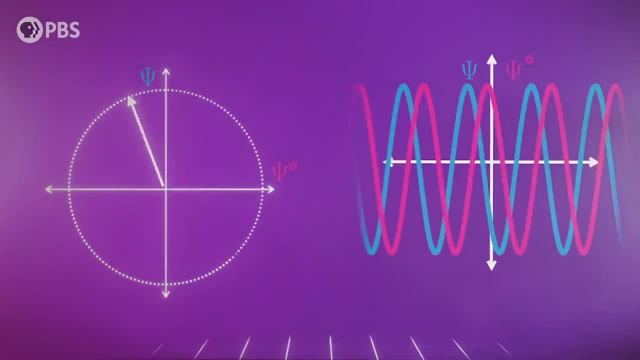 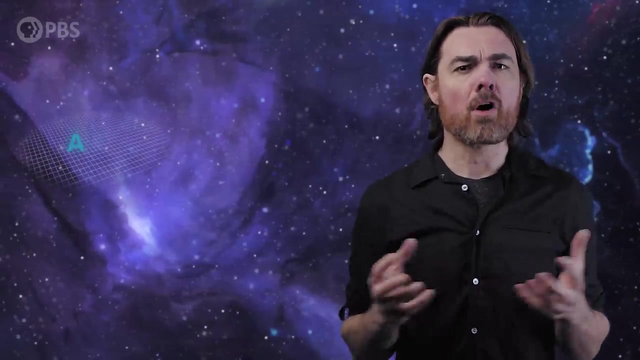 of freedom leads to a gauge field. We've seen an example of this. The exact phase of the quantum wave function from one point in space to the next local phase doesn't affect measurable quantities, Only relative phase matters. When we enforce this requirement, we find that we have to add: 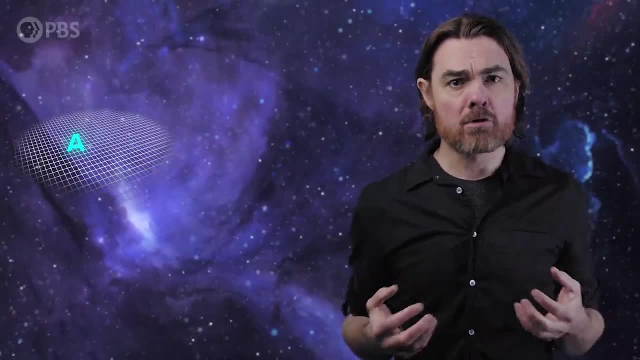 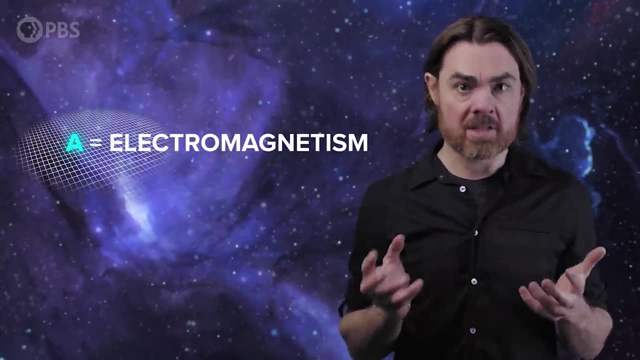 a new quantum field to the Schrodinger equation that lets the universe counteract these phase transformations. That gauge field turns out to be electromagnetism, And oscillations in this field are the photon, our first gauge boson and carrier of the electromagnetic force. 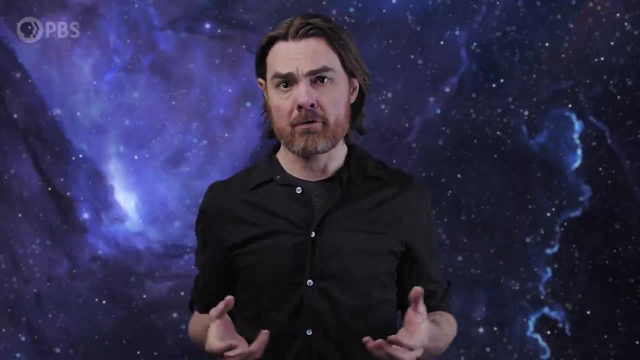 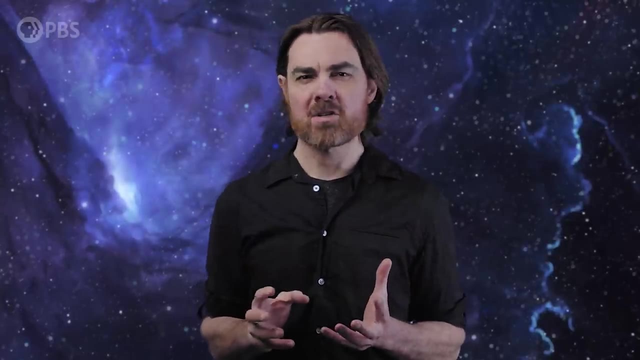 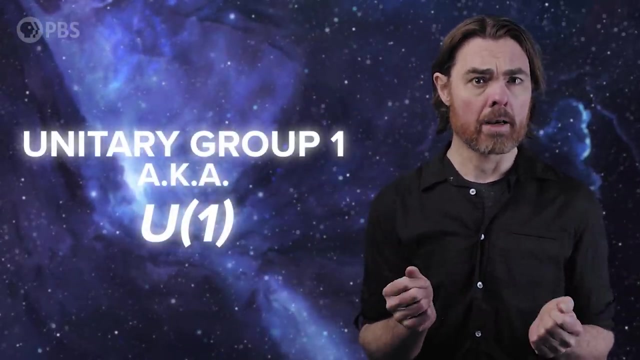 So one of the fundamental forces arises from a symmetry of nature, In this case the fact that the laws of physics are invariant under changes of local phase. The set of transformations that can change local phase are an example of a symmetry group, In this case unitary group 1, or U-1.. These transformations 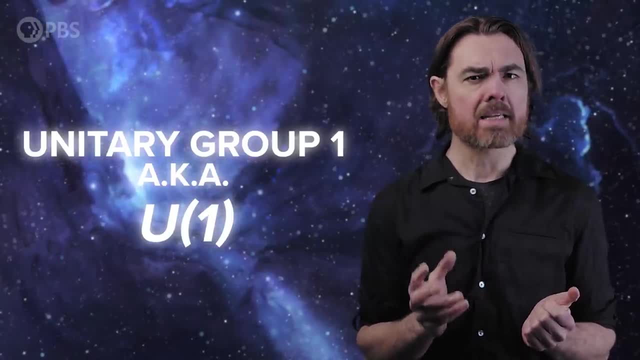 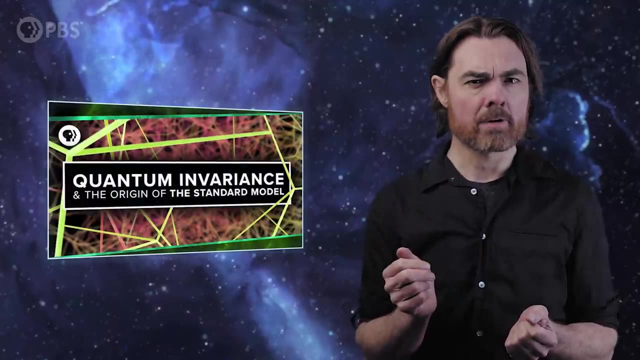 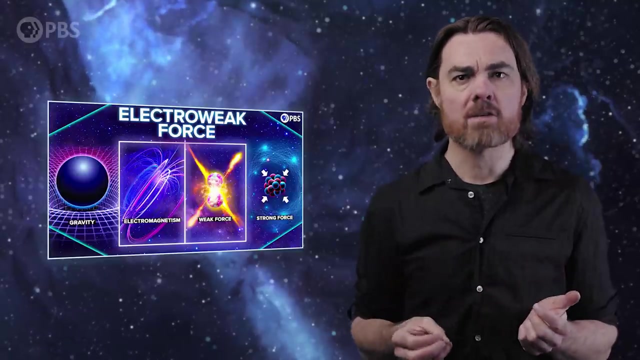 can be represented with just one number, in this case rotation of a phase angle vector of unit length. See this episode for all of the nitty gritty. this is just a refresher. In the next episode we tried the same trick to explain the weak interaction as arising. 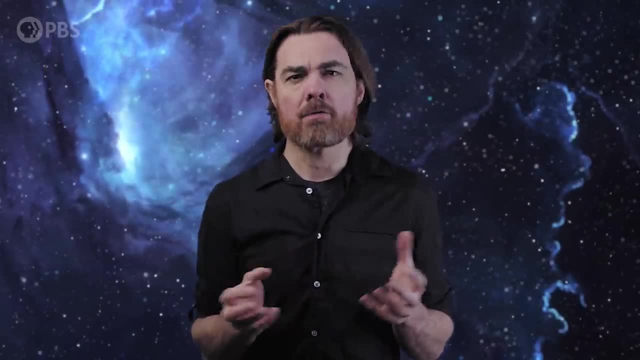 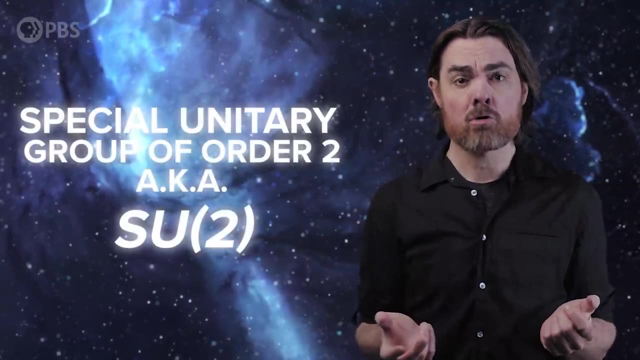 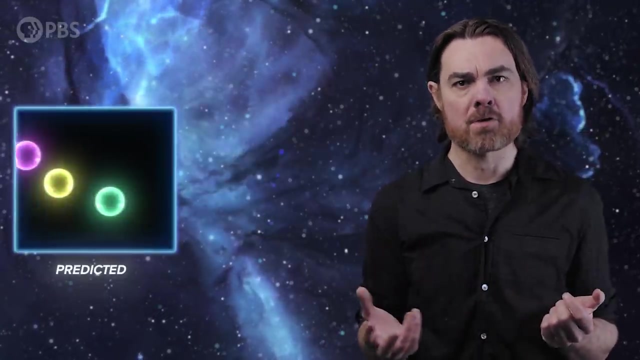 from symmetries, We saw that we could invent a pair of totally abstract degrees of freedom and demand that the universe be invariant to transformations of these. We call this symmetry group SU for reasons. That requirement gave us a new gauge field that had three force carriers that look awfully. 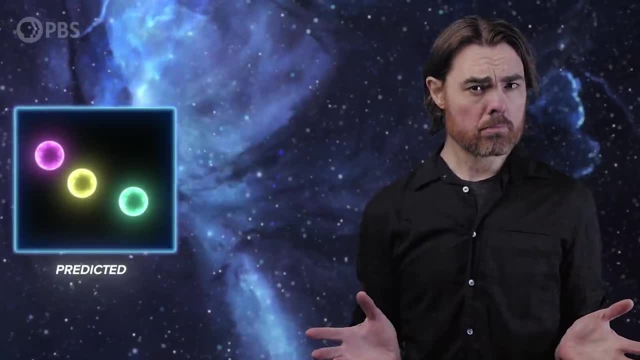 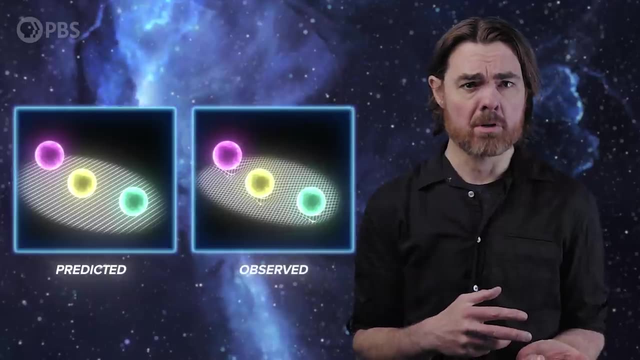 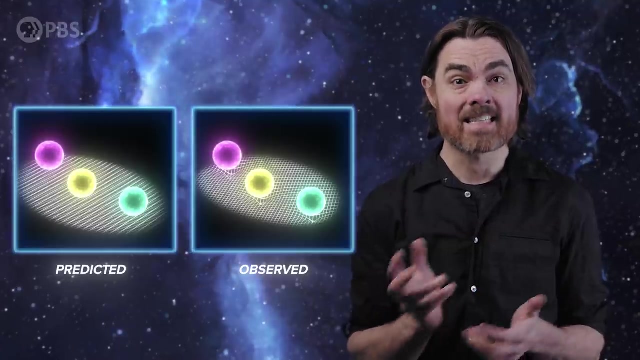 like the weak force bosons. So far, so good, Except that the predicted particles are massless, while the real weak force bosons are, as I mentioned, pretty hefty, And that is a huge deal breaker. actually, Massive bosons break gauge symmetries. 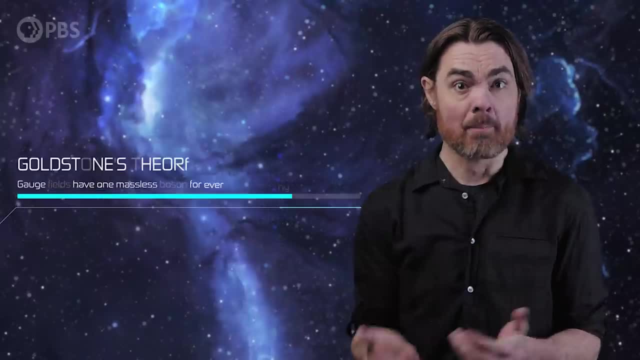 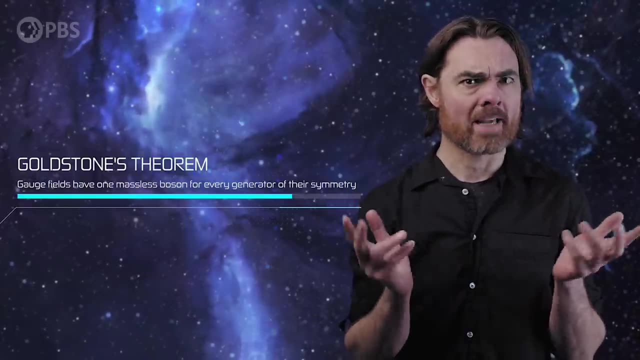 According to something called Goldstone's theorem, all gauge bosons are massless. So so far so bad, But we're going to forge on anyway and hope that this all gets sorted out. Another problem with this first pass at the weak force is that it has absolutely no connection. 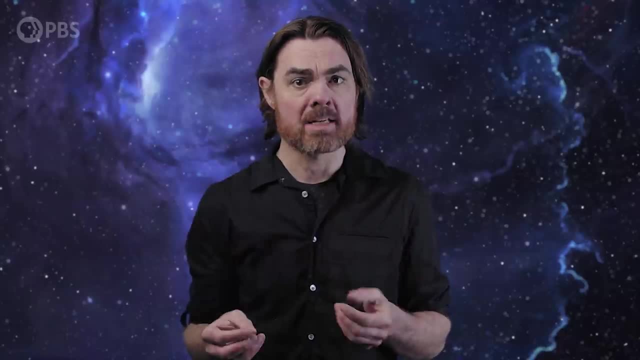 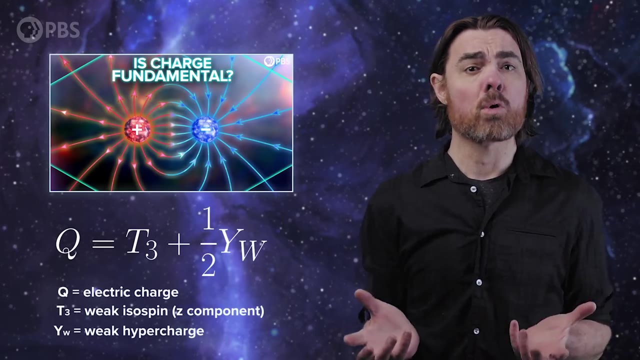 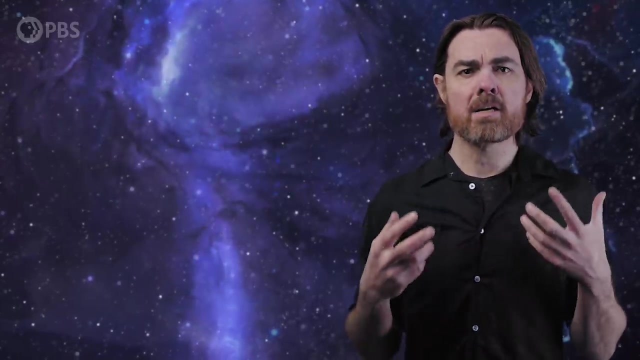 to electromagnetism. His bosons do have properties that look like weak isospin and weak hypercharge, but no electric charge. In our universe these three quantities are sort of locked together, Only taking on certain values. To see if we can duplicate that in our theory, we need to combine the U1 and the SU2 symmetries. 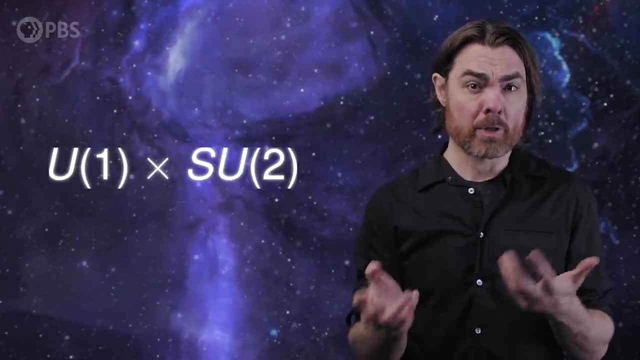 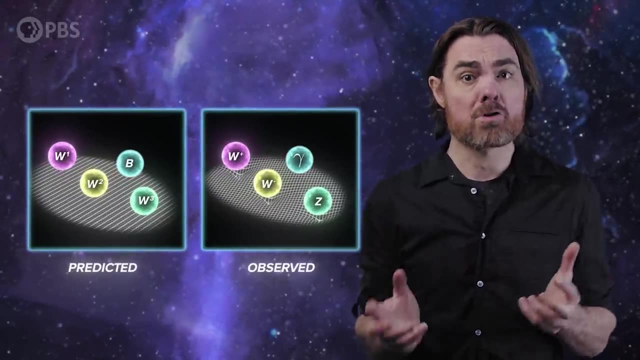 so that they all apply at the same time. We call this combined symmetry group U1, cross, SU2.. The resulting gauge field still has bosons that look a bit like the photon and the three weak force bosons, but the latter are still massless and the resulting charges are completely 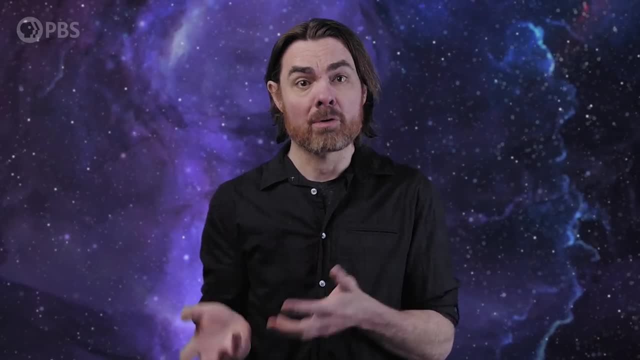 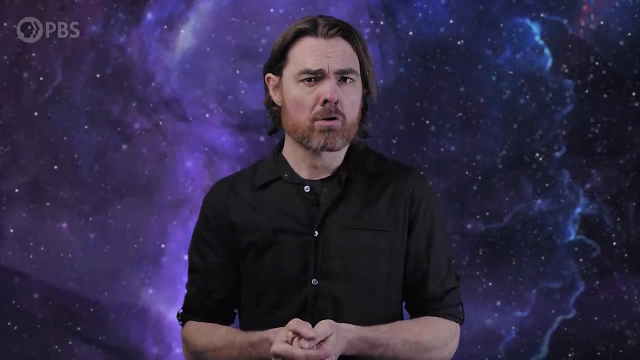 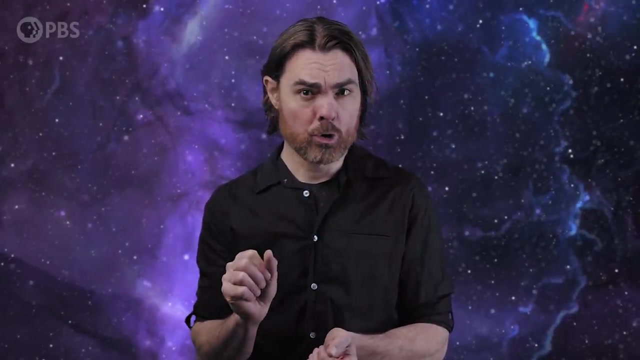 unconnected to each other. They're all free to be whatever they want, Unlike the real universe Where isospin and hypercharge are tightly coupled and their combination defines electric charge. So is it time to give up on this symmetry stuff. Well, there's one more long shot clue. 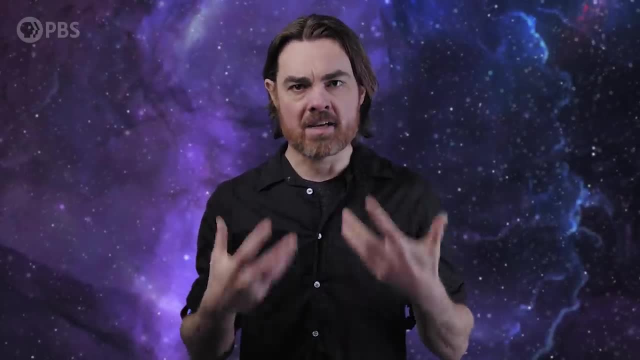 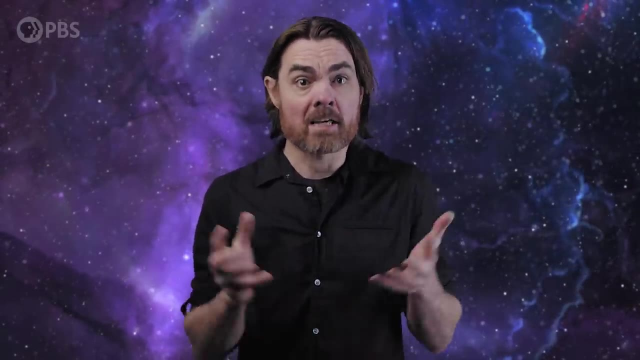 I said that massive bosons break the gauge symmetry. But what if that's okay? We've also talked about the idea of symmetry breaking before using this example of a bunch of bar magnets. These magnets have a very similar structure. They're not always the same. They all have high temperature which makes them move randomly. But as the system cools down, this random thermal motion gets overpowered by the magnetic interaction and they all end up aligning. The equations of magnetism don't start out with a preferred orientation, but in certain. 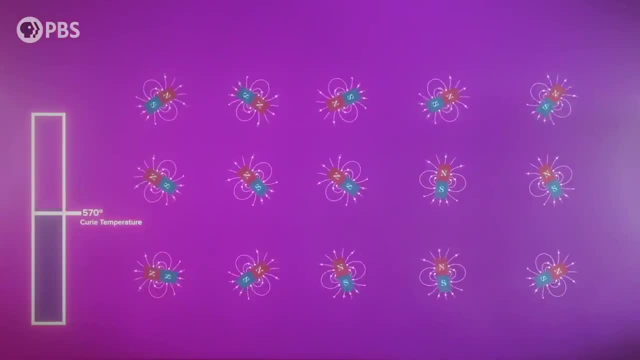 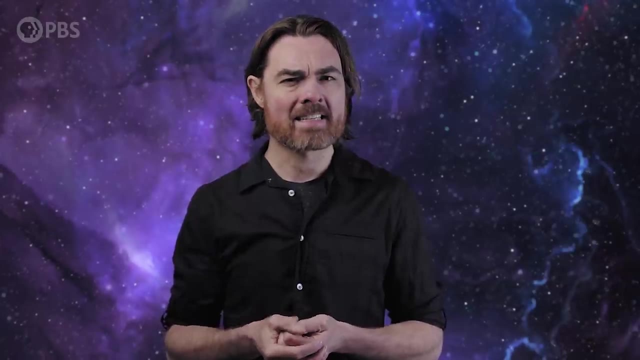 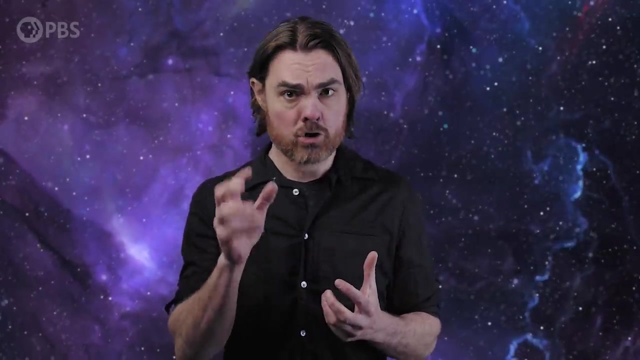 conditions, namely cold ones, the system chooses a preferred direction. This is an example of spontaneous symmetry breaking. so if a bunch of magnets can live in a state that violates our magnetic interaction- this would be a very common expression of violates the symmetries of their ruling equations- maybe the universe can too. 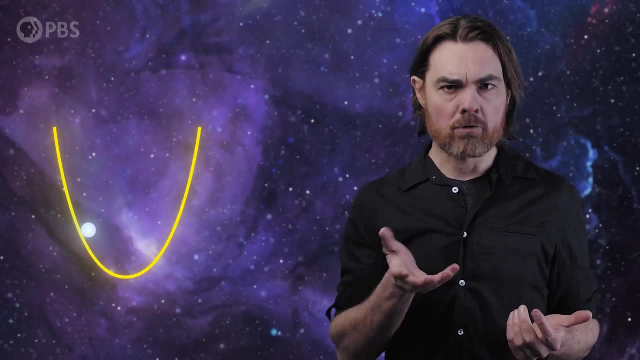 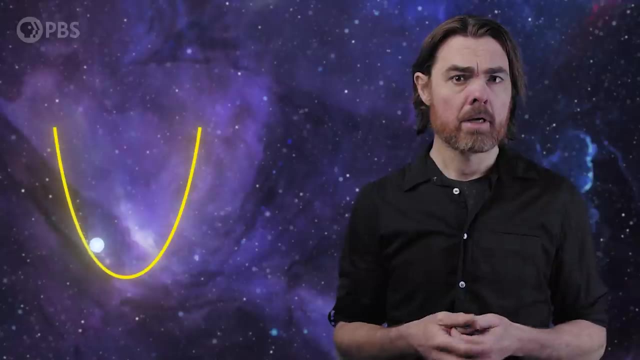 Here's another analogy: Consider a ball rolling back and forth in a valley. The equations describing its motion are symmetric between left and right, because the valley is symmetric. Now imagine it wasn't one valley, but two valleys, with a hill in the middle: The system. 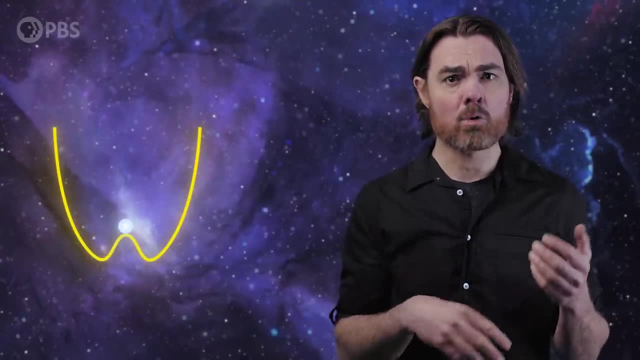 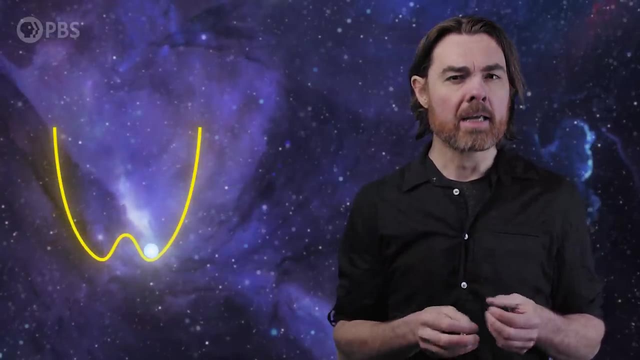 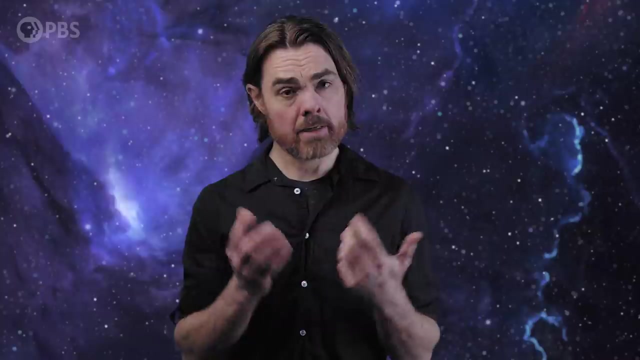 is still symmetric, but if the ball starts at the top of the hill, it will randomly roll down into one of the valleys. Now, the current state of the system has a broken symmetry, even if the symmetry of the landscape remains. Let's see if we can break the symmetries of the universe in a similar way. 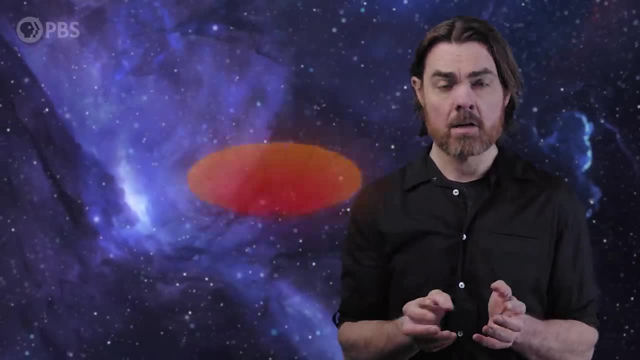 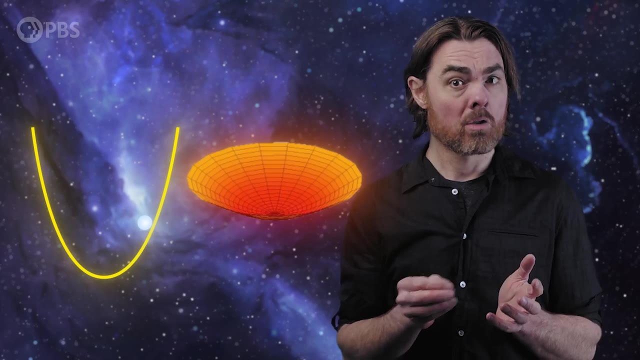 The equivalent of the simple valley does exist. A quantum field can oscillate around some zero-point value like a ball rolling back and forth in the valley. The walls of the valley are just the potential energy, the energy stored when the field moves in the 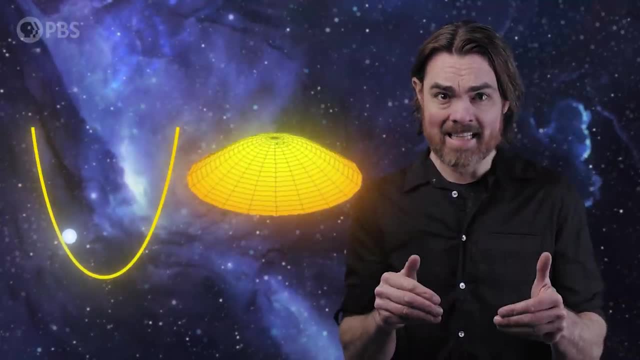 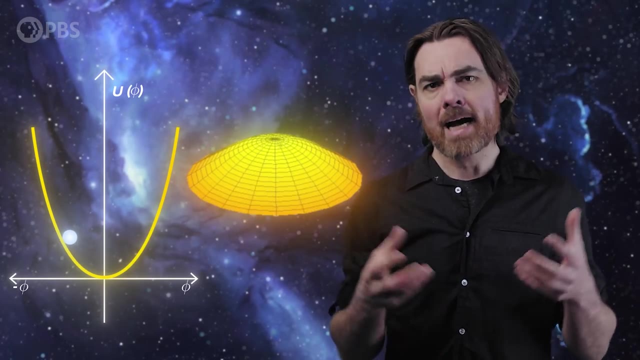 direction of the vertical axis. So it moves away from the zero point, trying to pull it back to the center. Graphing this, the vertical represents potential energy and the horizontal represents the field strength. Particles of the field are just oscillations of its field strength across. 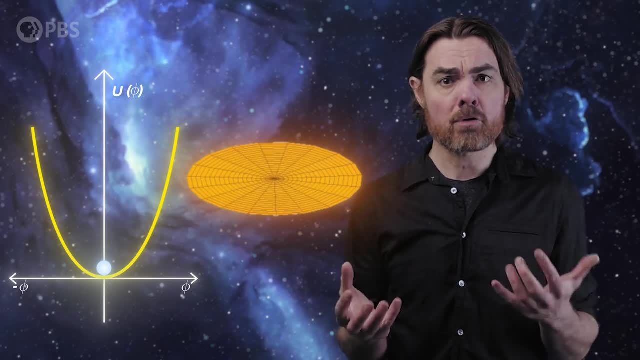 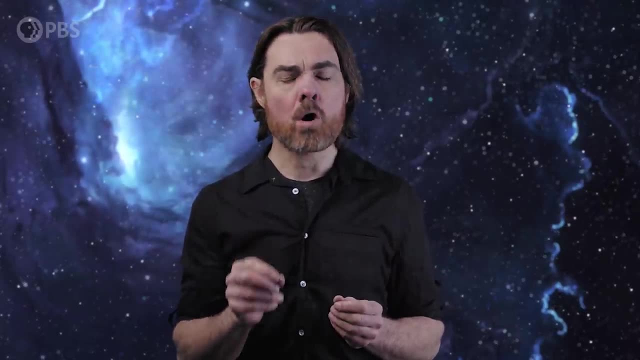 the lowest point, where the field strength is zero. But if there are no particles around and the field just sits at the lowest point, we call that the vacuum state. Easy stuff, right? In that case you won't mind seeing the math. 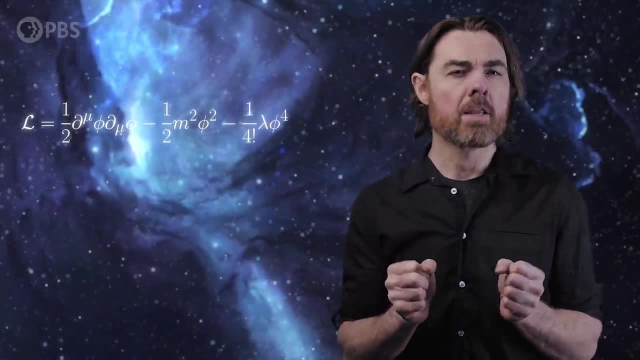 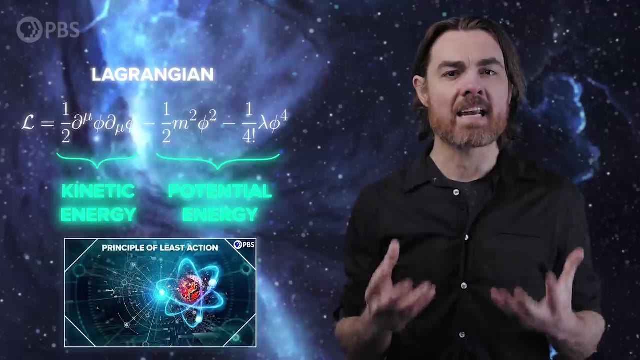 Don't freak out, it's not on the test. This is a Lagrangian, something we've covered before. It's really just the difference between the kinetic energy and the potential energy in the field. Our plot was of the potential energy part. 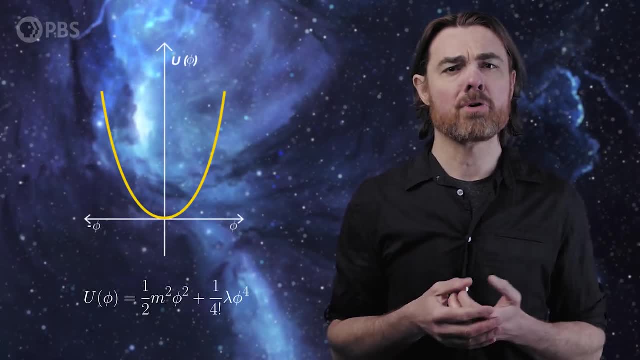 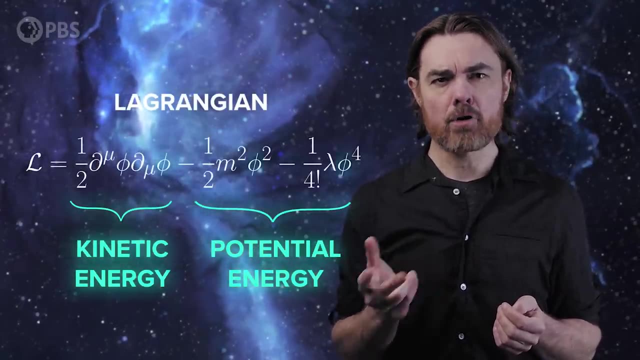 This particular Lagrangian describes a simple quantum field made of massive particles which interact with each other. Let me talk you through the hieroglyphics. Firstly, phi is the quantum field itself. It just means there's a numerical strength of the field everywhere in space. 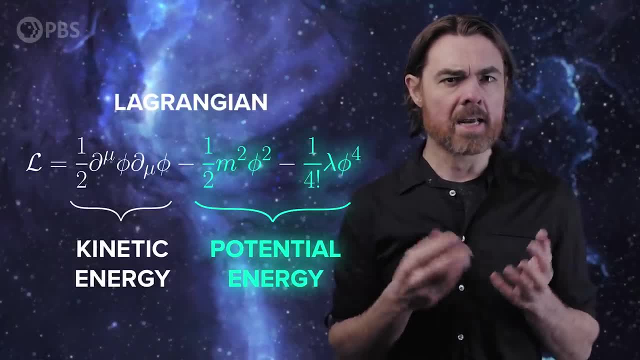 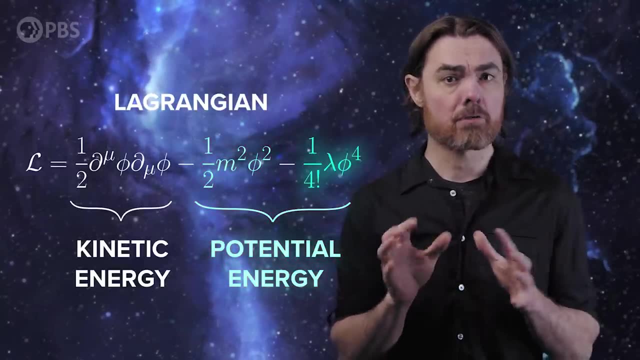 The potential energy part is the shape of the field and it's made of various powers of the field's strength, representing ways that the field's particles can interact. For example, this phi to the power of 4 term says that the particles of the field interact. 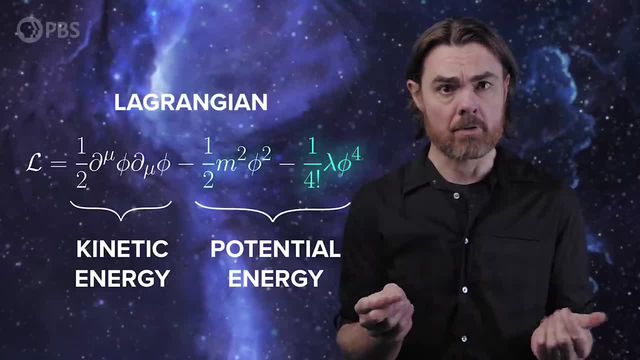 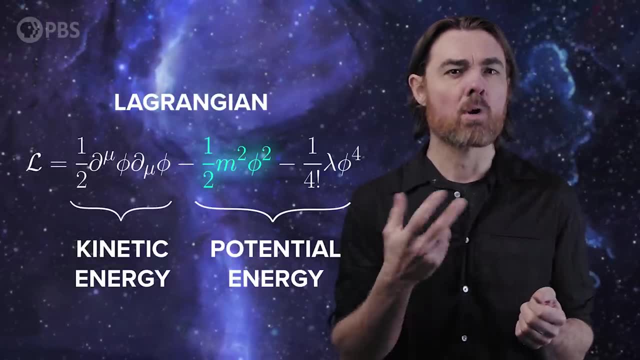 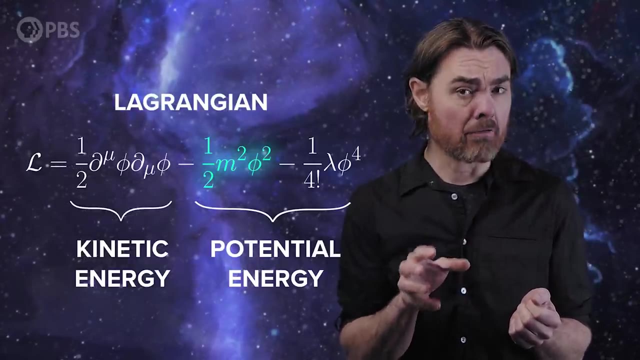 with particles of the same field with strength lambda. This phi squared term represents the field interacting with the field. That self interaction is what leads to the property of mass Gauge. fields shouldn't interact with themselves, so shouldn't have a phi squared term. 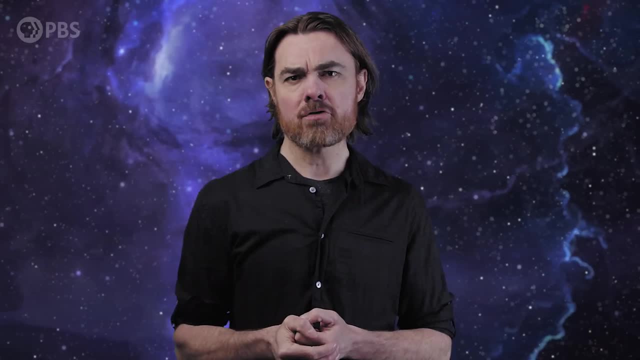 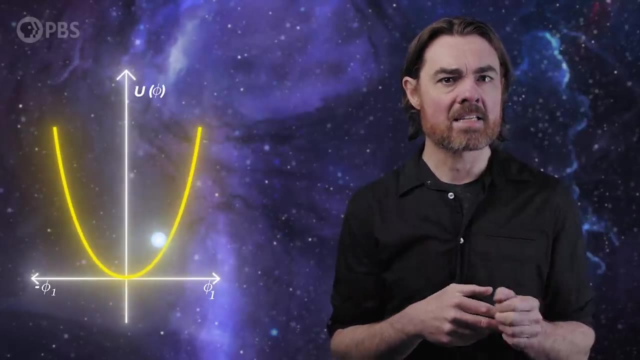 And that means this probably isn't a gauge field. The gauge field is a thing that comes from the degrees of freedom within this field. This particular Lagrangian has the simple symmetry that it's the same if you reflect it around the y-axis. 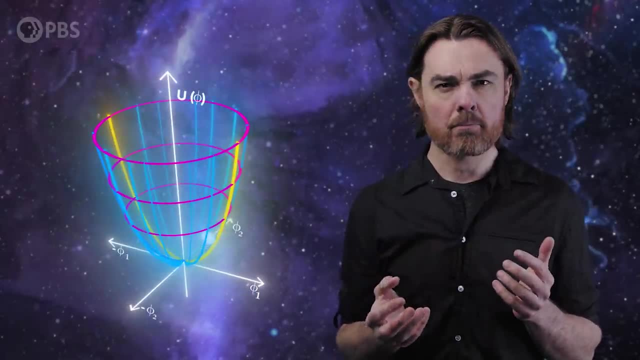 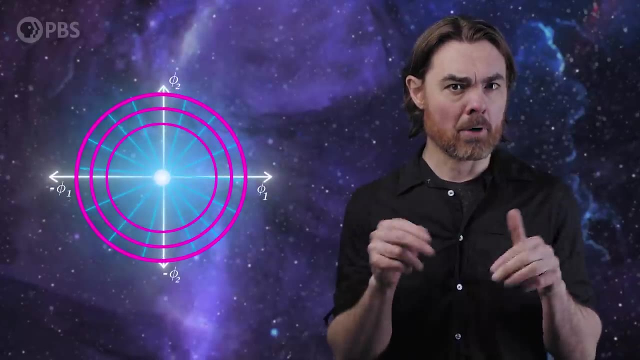 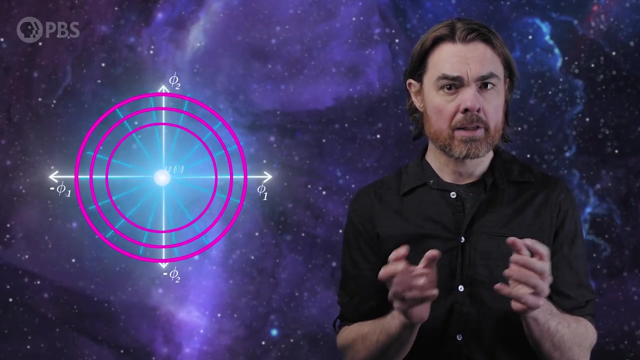 If we complicate things by adding a second field component, we're going to get a very complex field. If the current state of the field is at the bottom of the dip, then it has a single continuous degree of freedom in that you can rotate this thing and nothing changes. 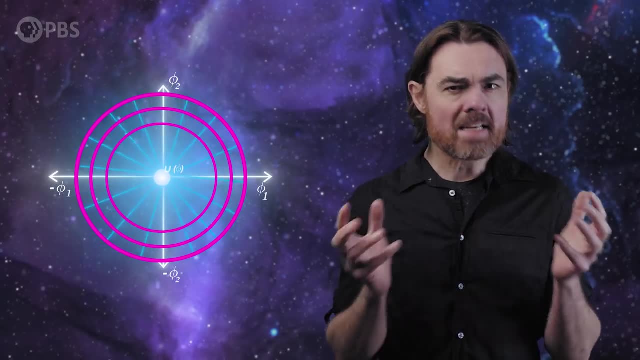 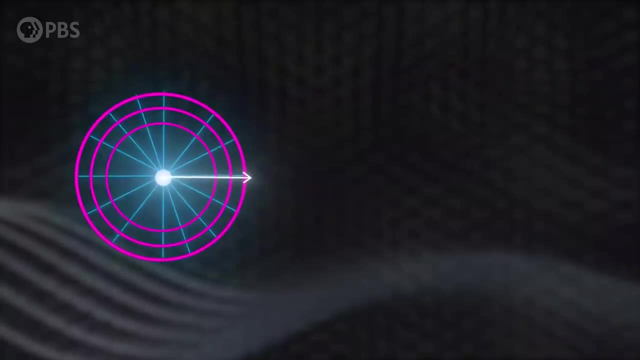 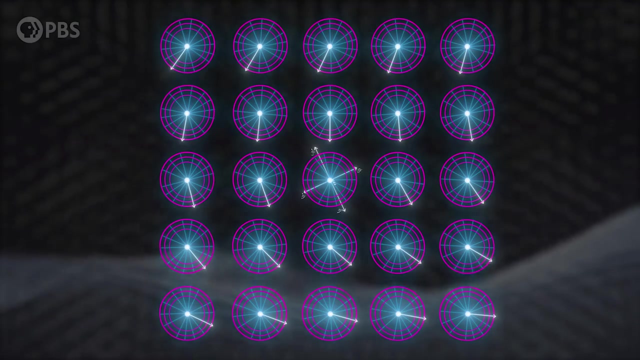 That would be a global U1 symmetry. Repeating our electromagnetism trick means requiring local U1 invariance. We need the laws of physics to still make sense if there are rotations from one point in space to the next. That means adding a new gauge field to the Lagrangian that allows the angle of this rotational. 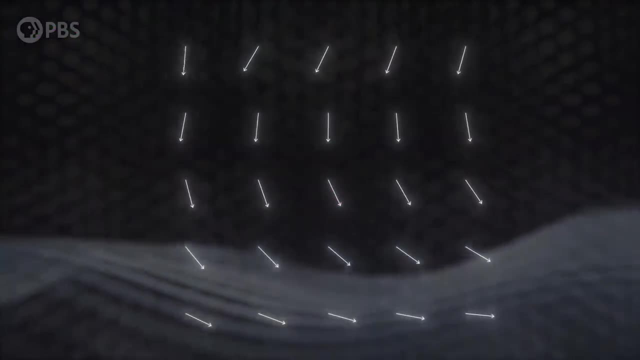 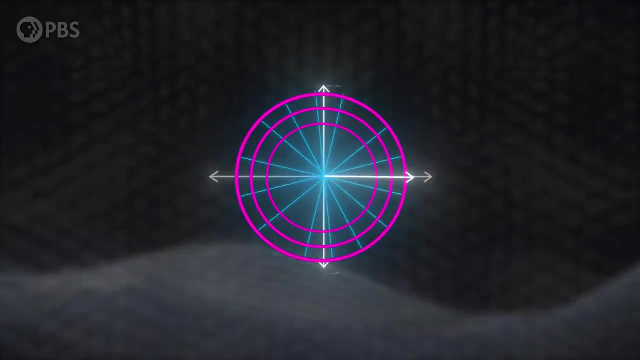 degree of freedom to vary. Oscillations in that field would be a gauge boson. You can think about those oscillations as the angle twirling around freely and it doesn't need any minimum energy to oscillate. so the gauge boson is massless. 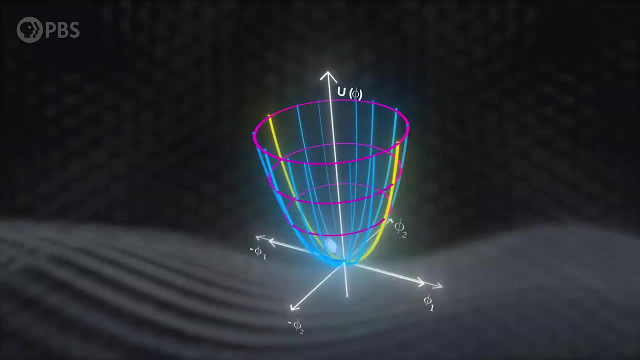 On the other hand, the particle of the original field needs a rest mass index. And since we've already got the original field, we need to add a rest mass index field to it. And if we add a new low- fragments field to the Lagrangian, that allows the angle of this. 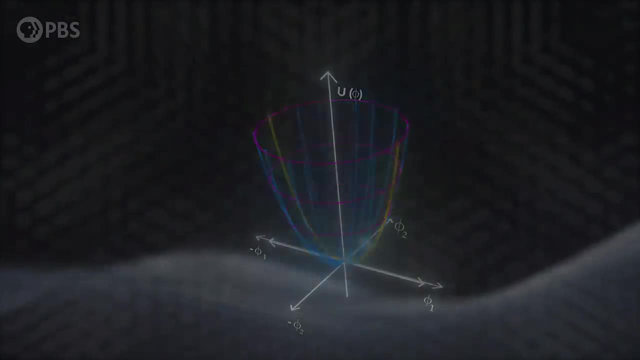 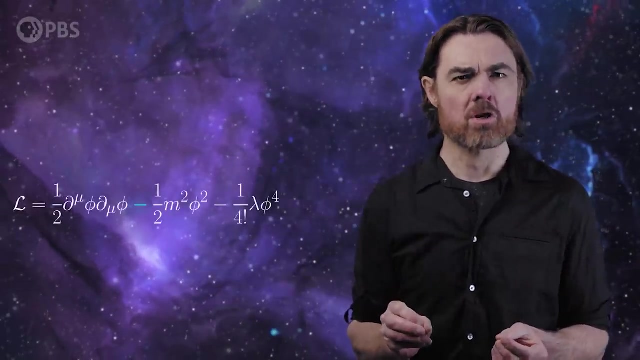 mass energy to be able to oscillate up and down the potential walls. So while this potential has its own mass of particles, it doesn't give us massive gauge bosons. Let's make a slight change. We're going to switch the sign in front of the mass term. 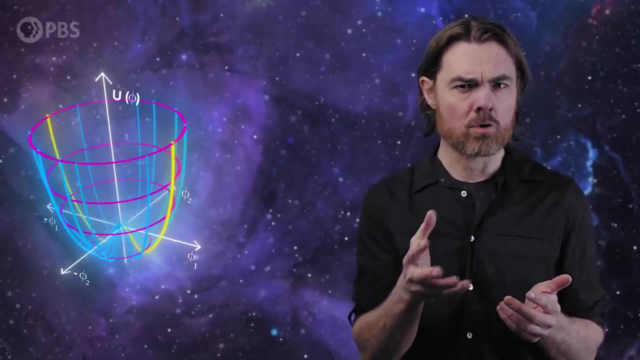 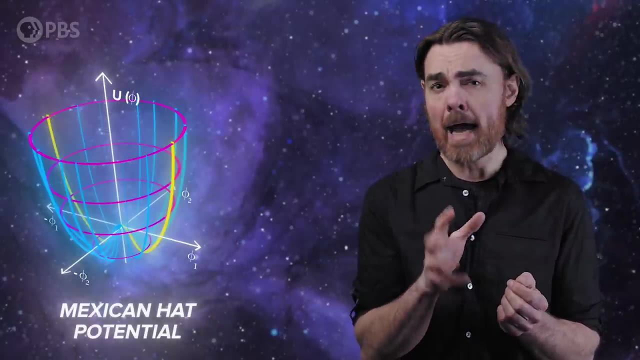 Then the potential would change to this, just like the two valleys we saw earlier. But now the second field component gives us this 3D shape. It's called a Mexican hat potential. This potential shape is the heart of the Higgs field. 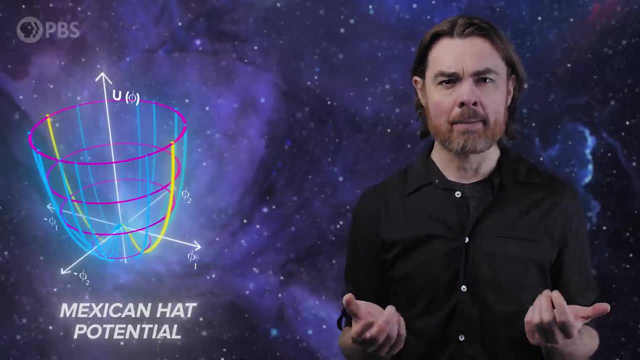 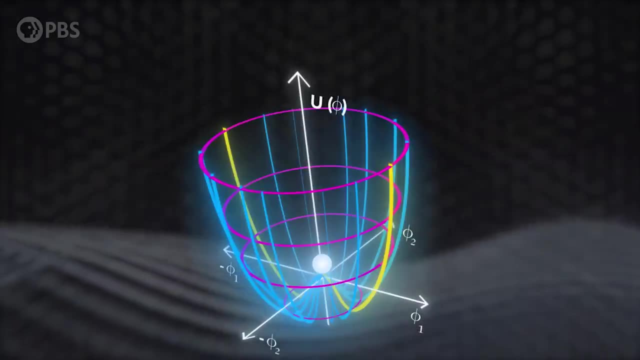 It's still a symmetric potential. It has the same global U1 symmetry as the original. But if the universe suddenly transitions from the old potential to this one, then we have a problem. The field's strength would find itself at the top of the little hill, but then quickly. 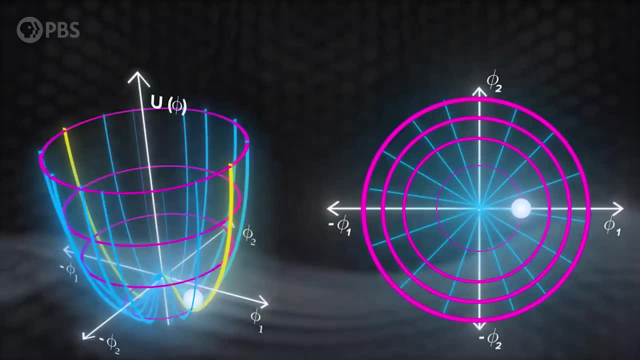 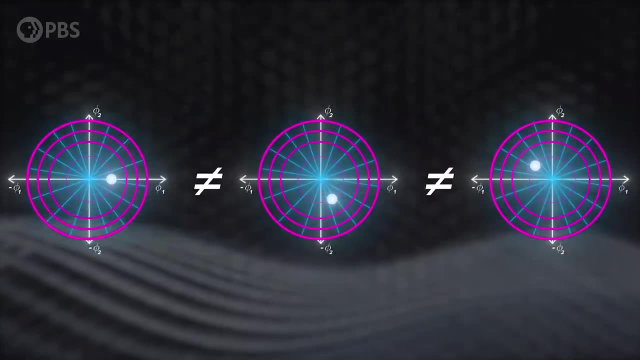 roll down in a random direction. The new state of the field would not be symmetric to the same rotations, because different points around this vector would be different. So the new state of the valley corresponds to different physical states. We say that the symmetry is spontaneously broken. 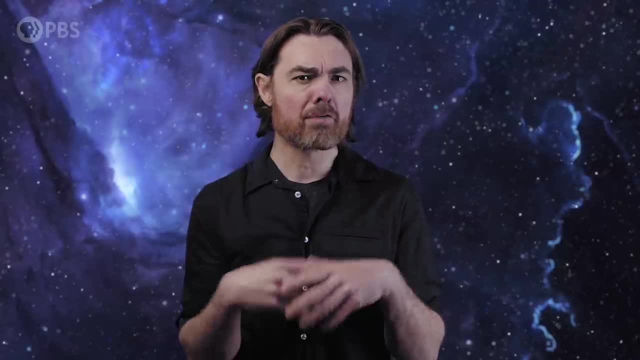 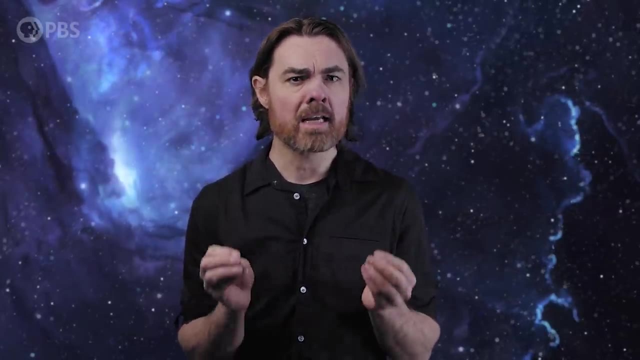 The current state of the field is a state of broken symmetry, even if the global field shape keeps its old symmetry. This is just like how the field of magnets can be in a state of broken symmetry even though the overall equations of magnetism have not changed. 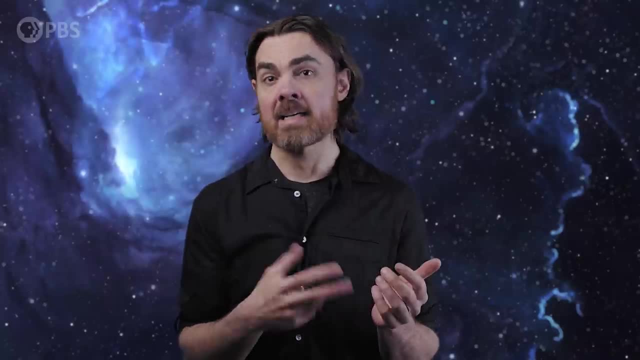 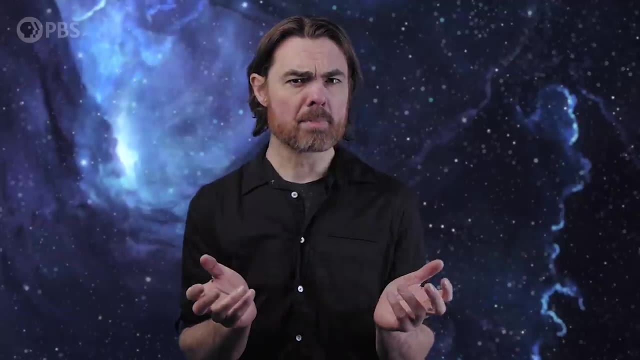 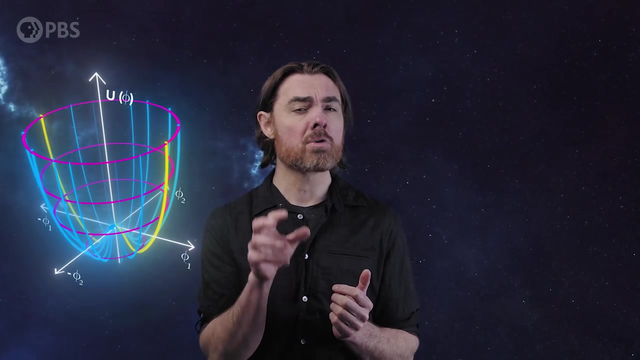 The transition from the central bump to the valley is an example of vacuum decay And we saw how this can lead to the creation of cosmic string. But cosmic strings are perhaps the least interesting part of this process. Once the field has reached the base of this new minimum, we have a new, stable vacuum state. 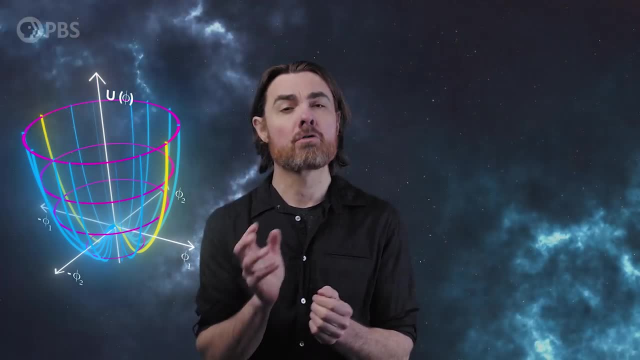 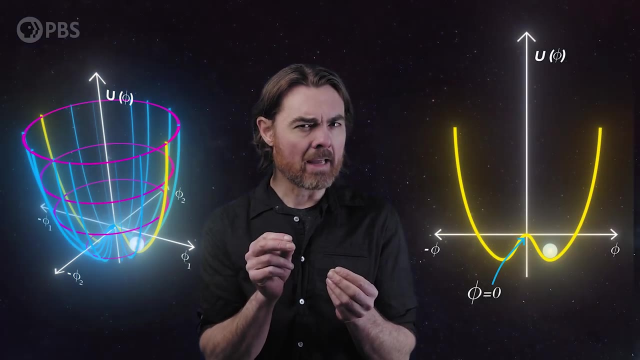 But this state is very different from the original for two reasons. The first is that the lowest energy state, the vacuum state, isn't where the field strength itself is zero, So this is called a non-zero vacuum expectation value. The original mass of the vacuum state is zero. 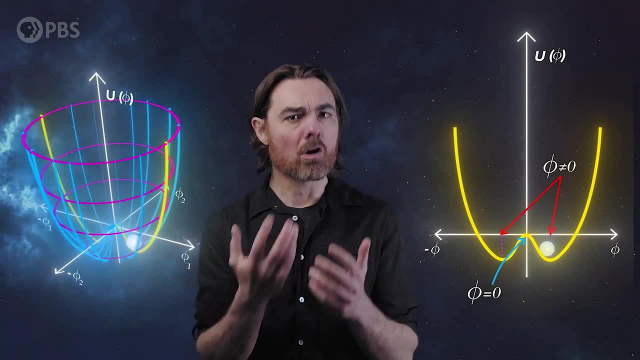 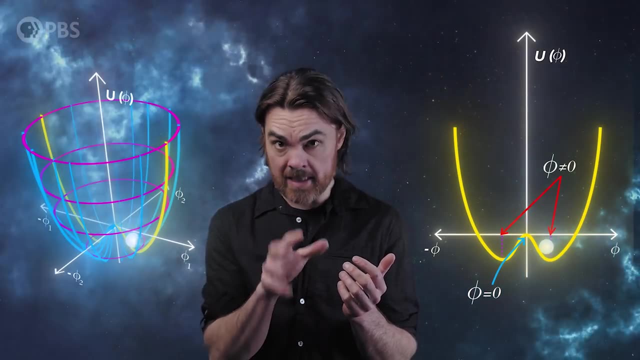 So the vacuum state is zero. The original mass of particles of the field now oscillate in the radial direction, but no longer centered on the zero field value. And this is the Higgs boson. The second weird thing: there's not just a single vacuum state, there's a ring of 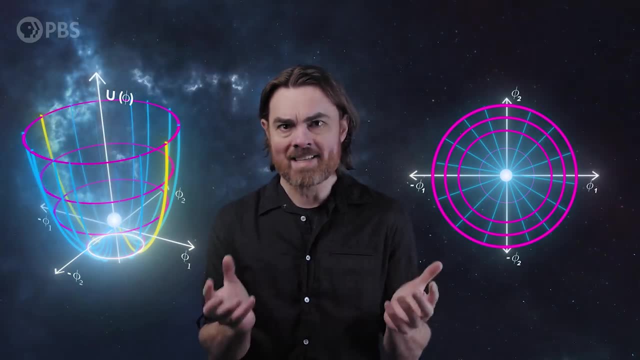 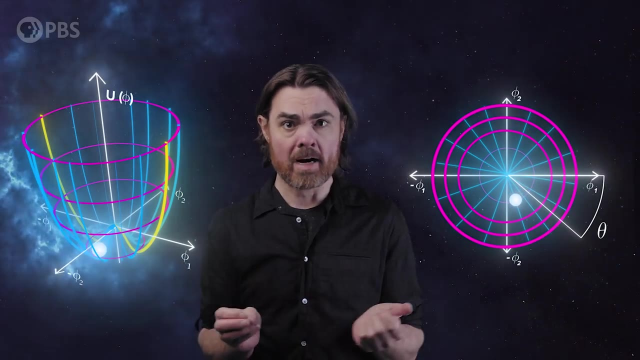 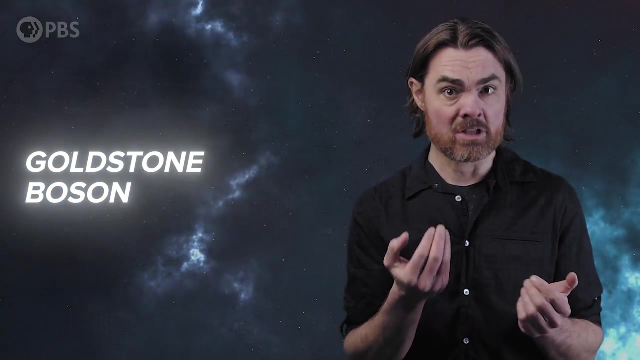 valid states. The universe will just have chosen one state randomly, But the field can also oscillate along the base of the valley in what we'll call the theta direction. The resulting particle is called a goldstone boson And it's massless because the valley is flat. 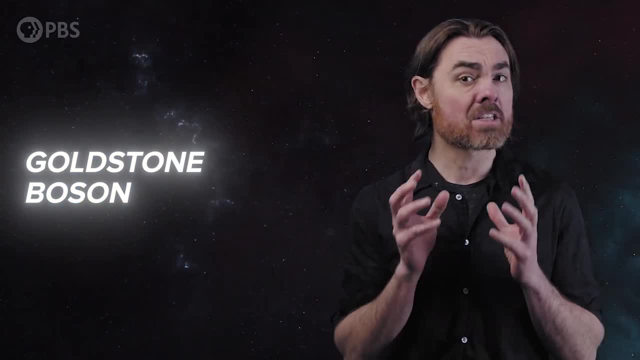 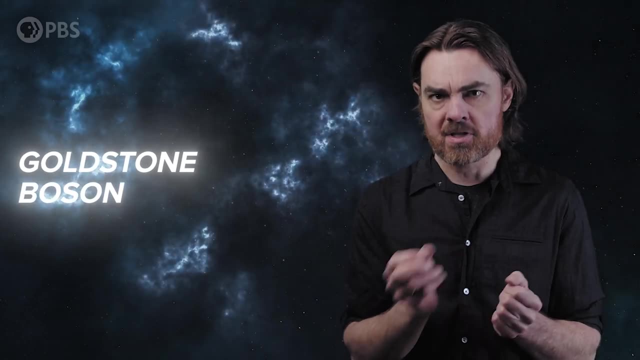 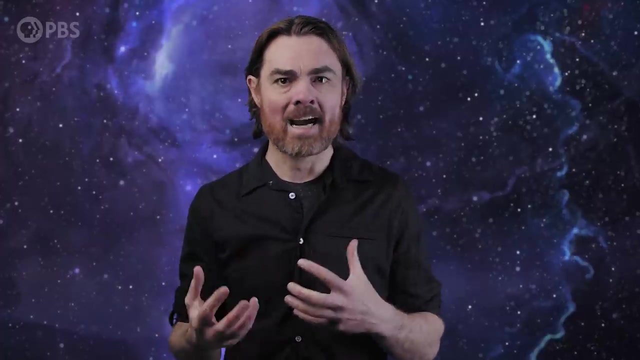 There's no energy differential. However, this is not a gauge boson, because location around the valley represents a real physical difference in the field state. OK, let's bring all of this together. We want to combine the weak and electromagnetic interactions, So we need simultaneous local U1 and SU2 symmetry. 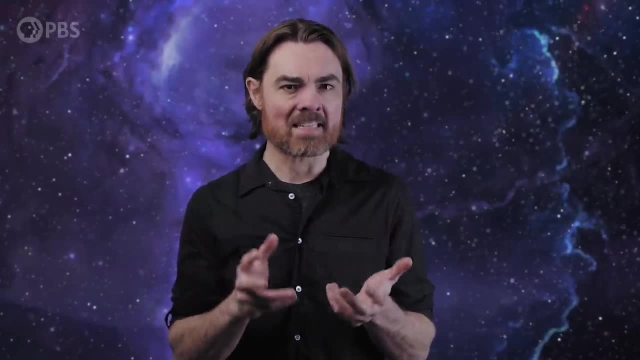 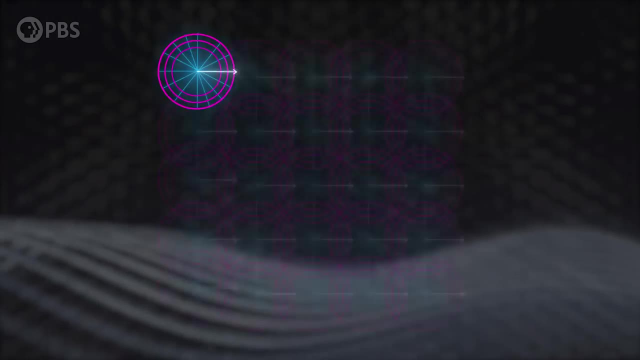 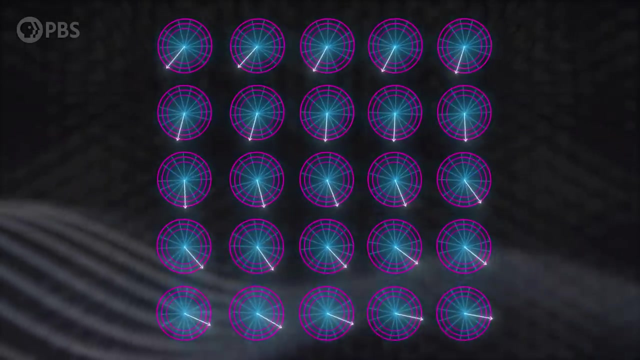 Let's just do U1. Because that gives us the basic picture, Because the potential is the same all around the valley. it shouldn't be possible to tell where in the valley you are. It matters if two adjacent patches of the universe are in different parts of the valley. 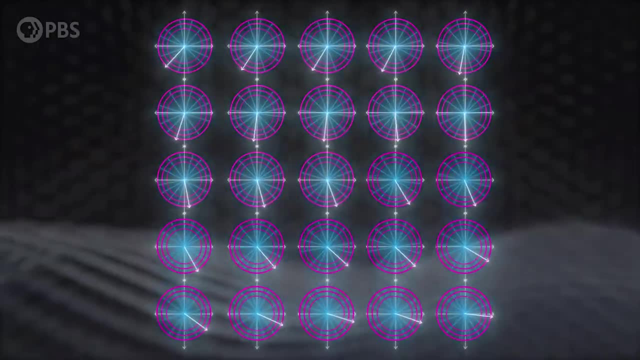 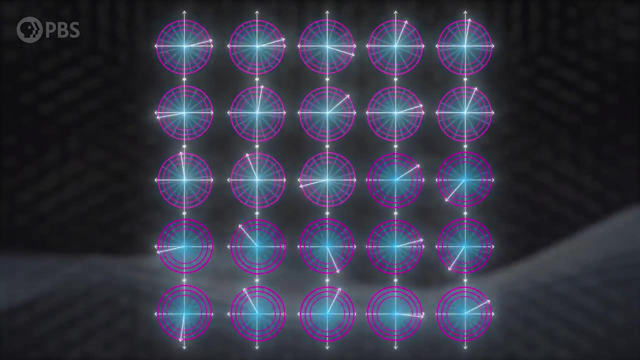 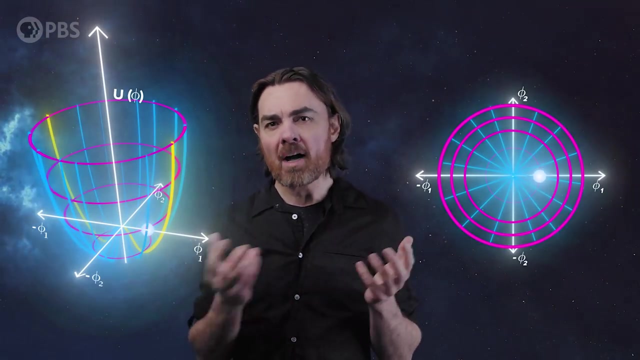 The relative difference in the angle. theta matters but exact values don't. So we're going to demand local U1 invariance and come up with a gauge field that shakes out the shifts in our arbitrary choice of the zero point of theta. But now this gauge field finds itself in a much more complex Lagrangian with this Mexican. 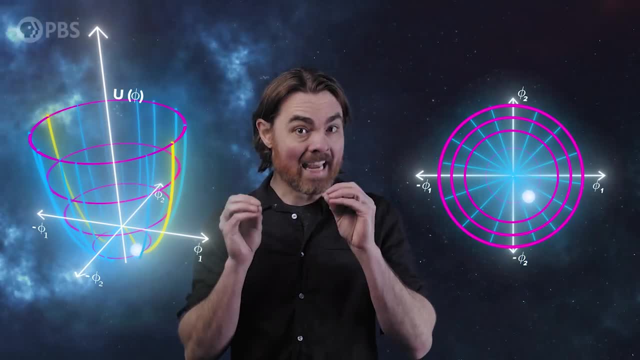 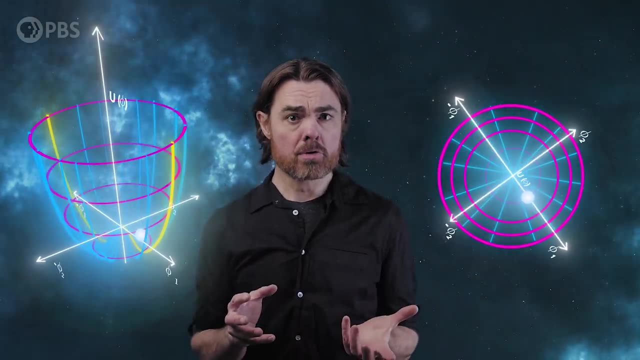 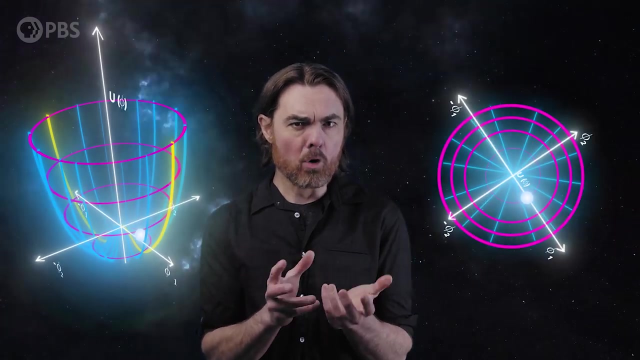 hat potential. Weird stuff happens when the gauge field couples to the particles of that potential. First of all, we see that the goldstone bosons, which are just oscillations in the theta angle, can be absorbed into this U1 gauge field. 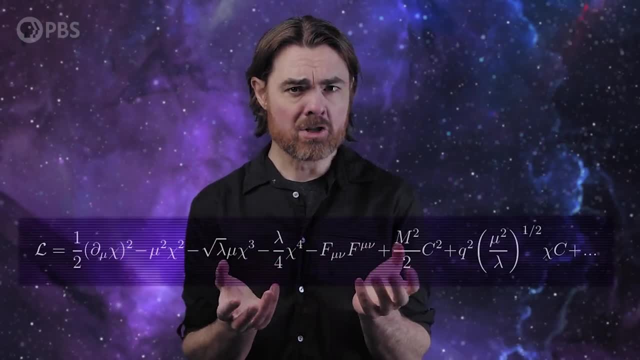 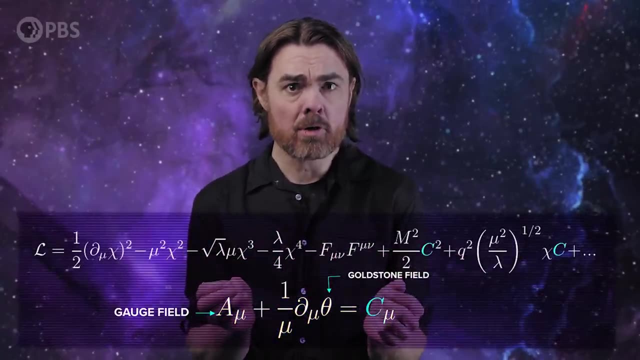 Both are oscillations around the valley In the Lagrangian they get lumped together into a single field. That's what we want. We want a single field term that still looks like a gauge field with a single gauge boson. The gauge field sort of eats the goldstone boson. 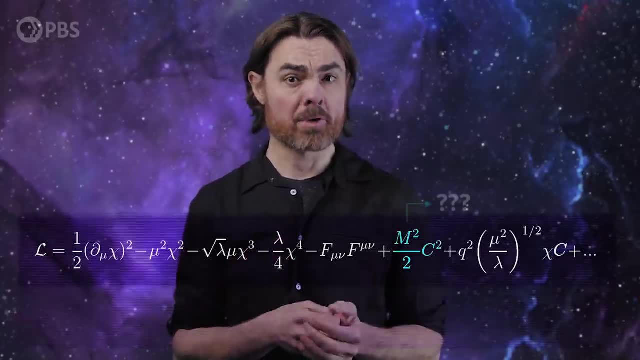 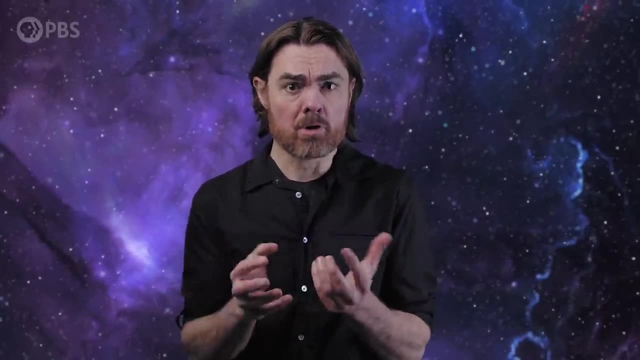 But when we do this, the new combined field has a field squared term in the Lagrangian, which is weird because those are mass terms, Except that neither the original gauge boson nor the goldstone boson that it just ate had any mass. 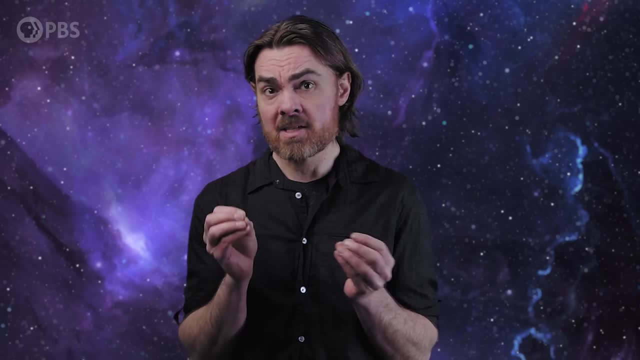 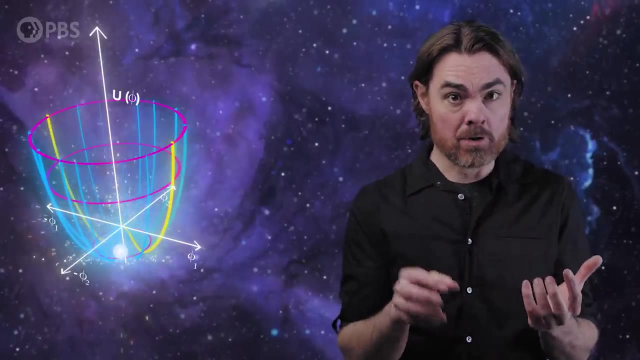 So where does this mass come from? Ultimately, it's because the gauge boson is now anchored to the Higgs field. So where does this mass come from? The goldstone boson that is now part of the gauge boson is coupled to the Higgs field. 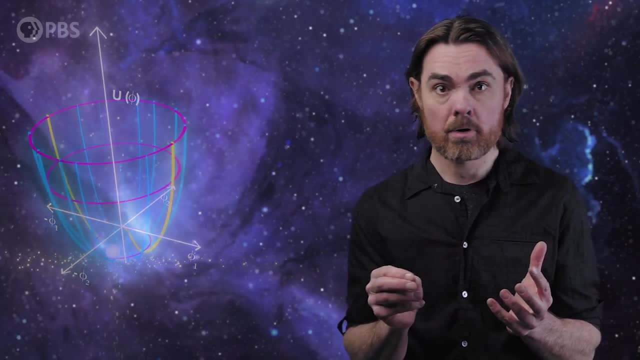 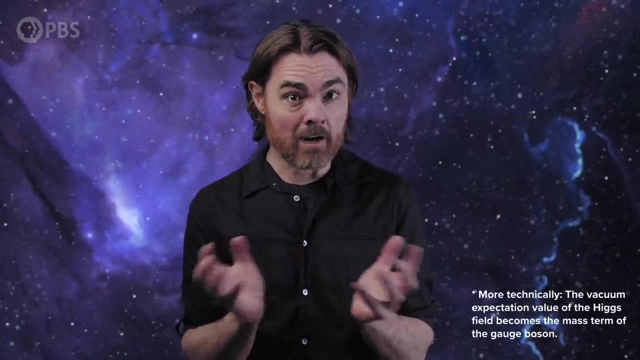 and that means that the gauge boson is also so coupled. Ultimately, this happens because of the non-zero vacuum state of the Higgs field. That little bit of Higgsiness everywhere refuses to cancel out in the Lagrangian, giving us our mass term. 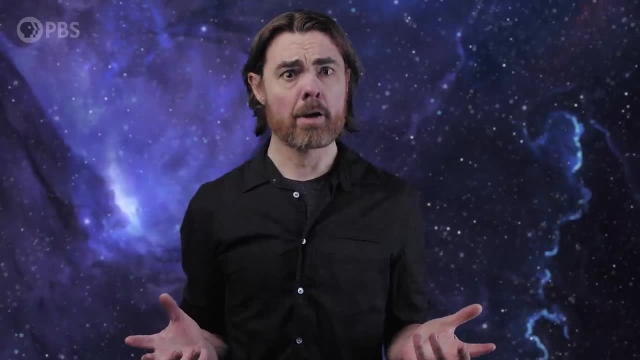 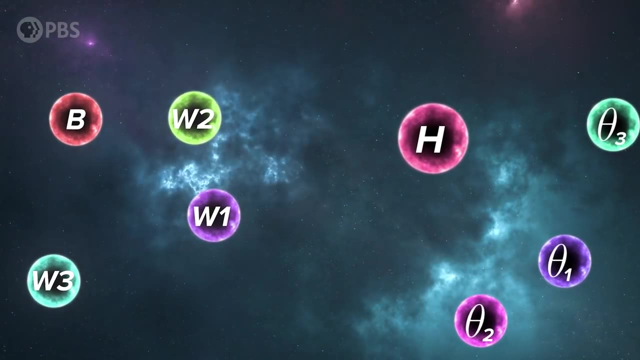 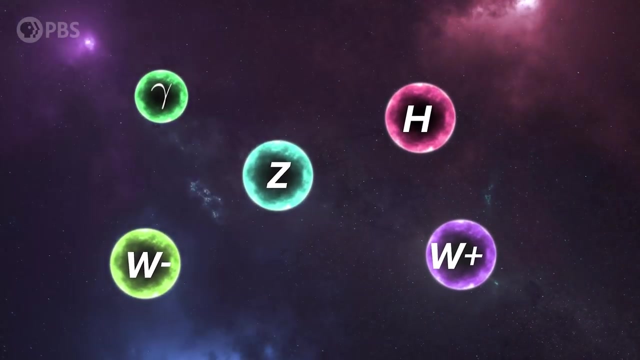 All of this was a simplified explanation. I know horrifying right Imposing the full electroweak U1 cross, SU2 invariance on the true Higgs potential gets you three goldstone bosons that are eaten by three of the four electroweak gauge bosons. 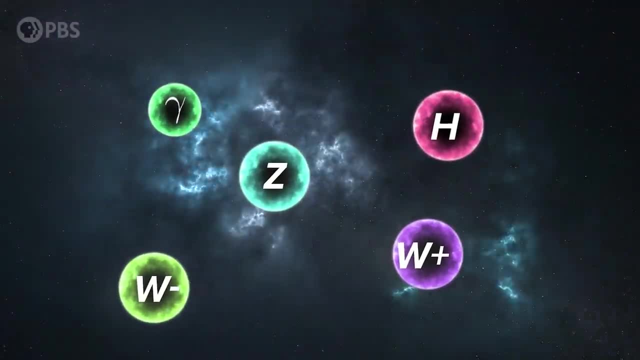 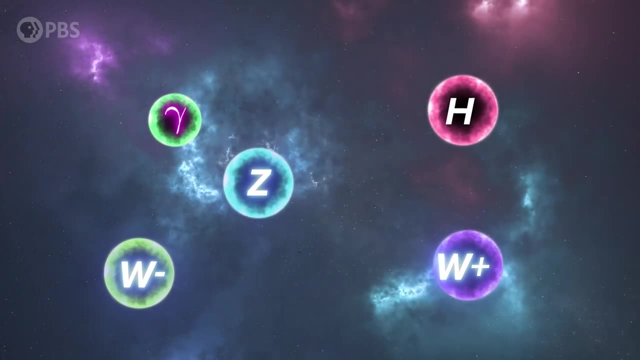 Those gain mass and become our 2W bosons and 1Z boson. of the weak interaction, The fourth boson manages to escape unscathed and massless, becoming the photon that we know and love. It flew free of its heavier cousins. 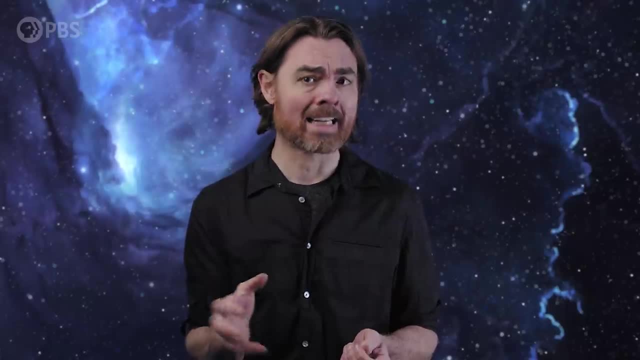 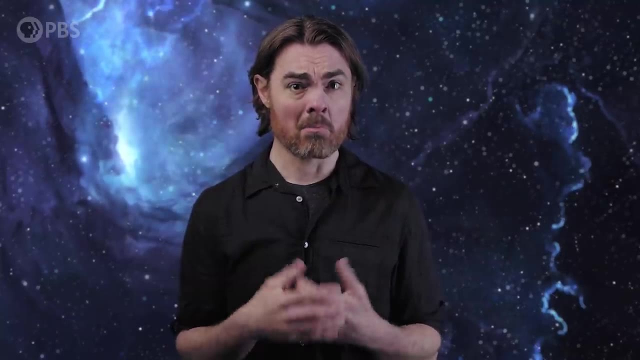 The independent mediator of the Higgs field. The Higgs field is now a mass term. It is a part of the old electroweak field, what we now experience as electromagnetism. While the W and Z slog on through the mire of their coupling with the Higgs field, their 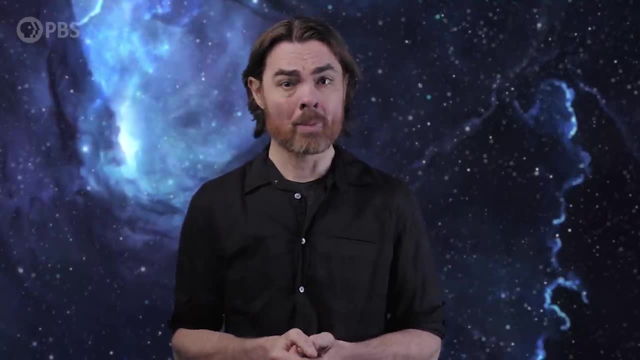 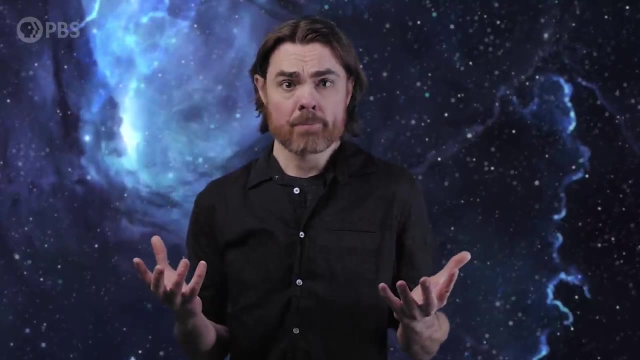 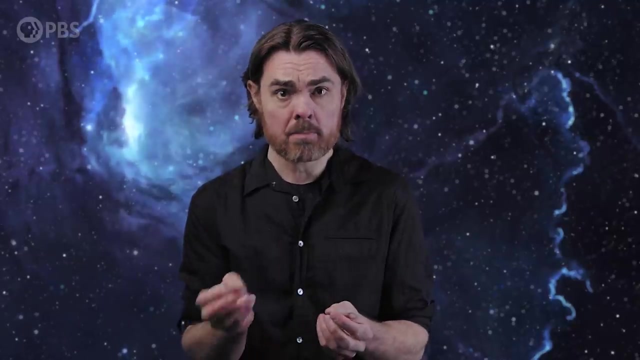 mass shortened their lifespans and so enormously reduced their range, weakening the force that they mediate. So that's where we are today. This is the Higgs mechanism. The Higgs field also gives mass to the matter: particles, the fermions. 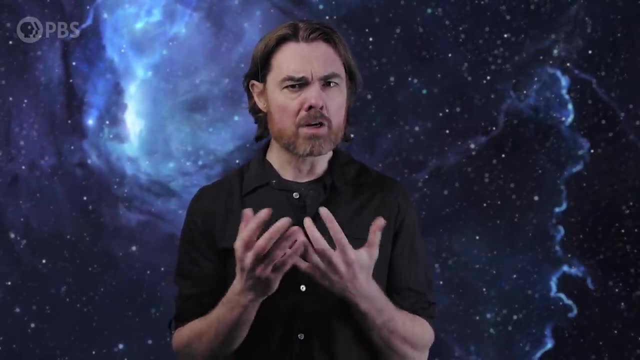 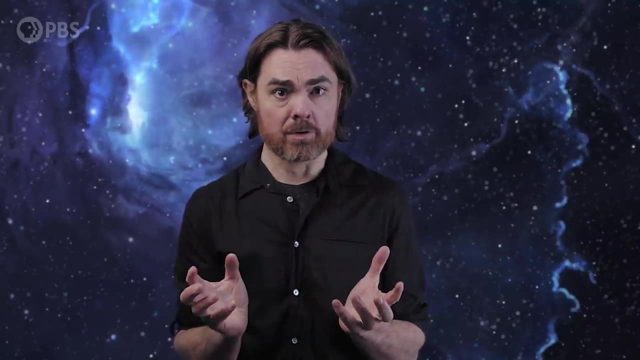 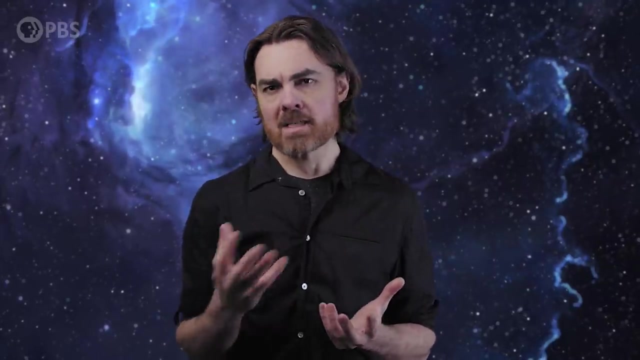 But that is for another time. But what about this new measurement of the W boson mass? Well, mass results from interaction with the Higgs field, but also from other subtle interactions that a particle can undergo. The predicted mass of the W boson takes into account all standard model particles that 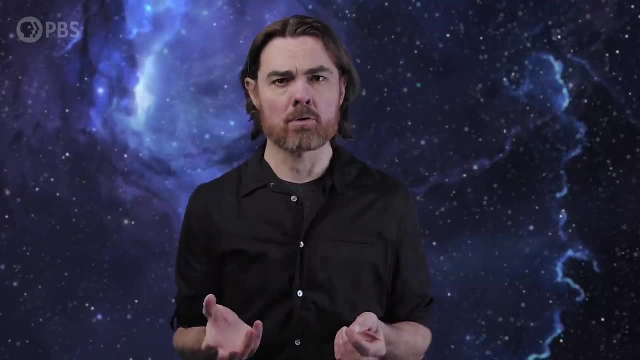 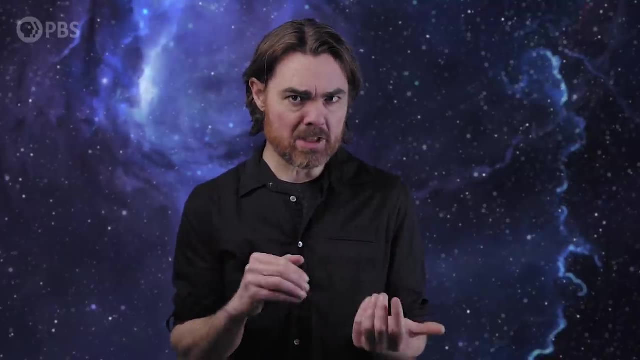 could have a ghostly presence as virtual particles in the energy field of the boson. The fact that Fermilab measured a mass of the W boson with the Higgs field is not a big deal, And a larger mass than was predicted suggests an unknown particle or particles flickering.